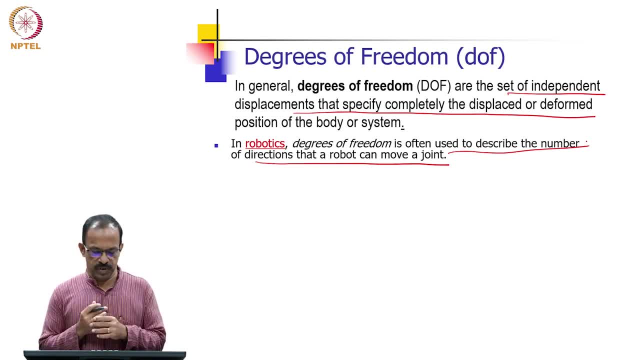 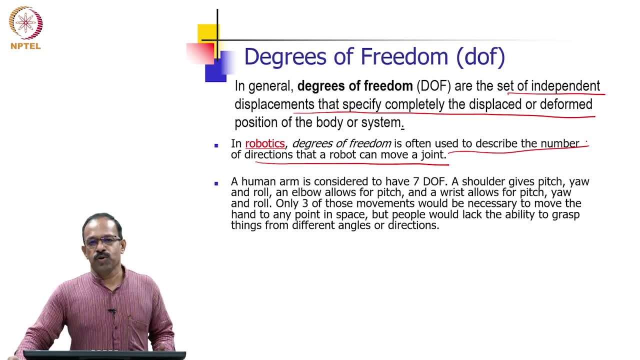 move in one direction, then we call it as four degrees of freedom, robot like that. So that is the way how it is defined. Now, as you know, human arm has got seven degrees of freedom because we have three joint motions here at the shoulder and then we have three joints or motion or three independent motion. 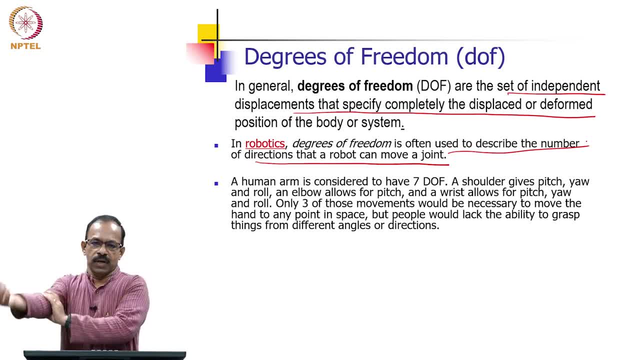 possible at the wrist and we have one at the elbow here. So we have, like this, seven degrees of freedom for our human hand. So we can call this as the pitch yaw and roll of the shoulder. So pitch yaw and roll of shoulder and elbow allows for pitch and wrist allows. 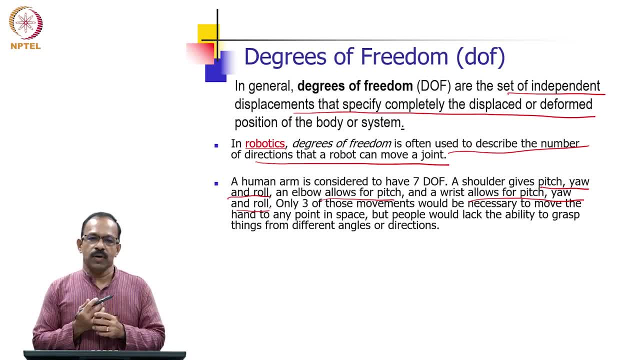 for pitch, yaw and roll. So all of us know that we can actually use these three joints to position the wrist at any point. So we can actually move this here and then in any plane. So we will be able to position the wrist in the space using the first three degree. 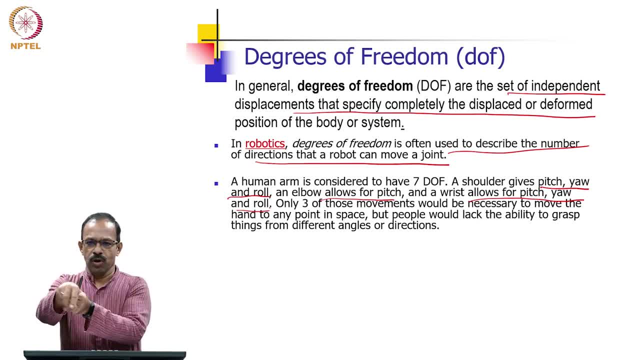 of freedom, Then the next three degrees of freedom can be used for orienting the tool. So I have a tool like this, So I have a tool like this for orienting it in the space. So three of these movements would be necessary to move the hand to any point in space. and if you do not have the 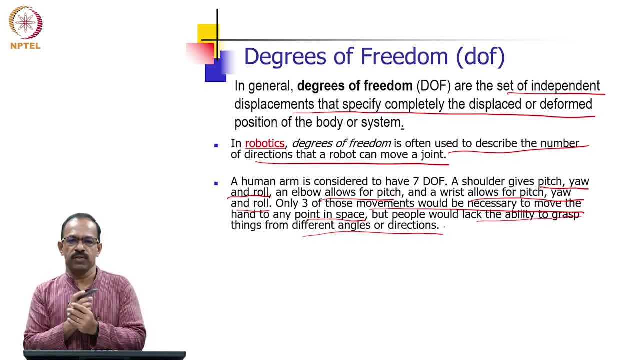 other things you will be. if you want to have it in different angles, then we need to have the orientation. That is the way how this three plus three works for positioning and orientation. Now, if a robot that has mechanisms to control all six physical degrees of freedom, 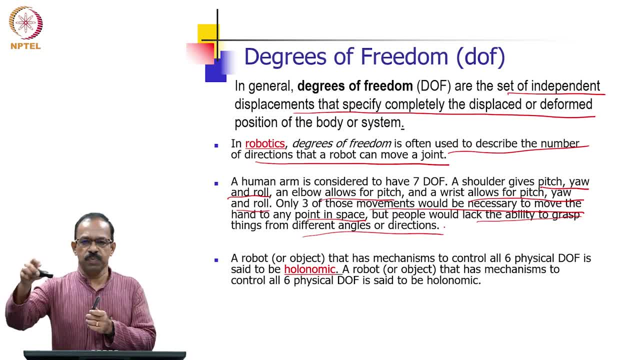 is said to be holonomic. That is normally. any object in space has got six degrees of freedom. So if we can actually provide six degrees of freedom for the robot to control all these, then we call it as a holonomic one. So that is the way how it. 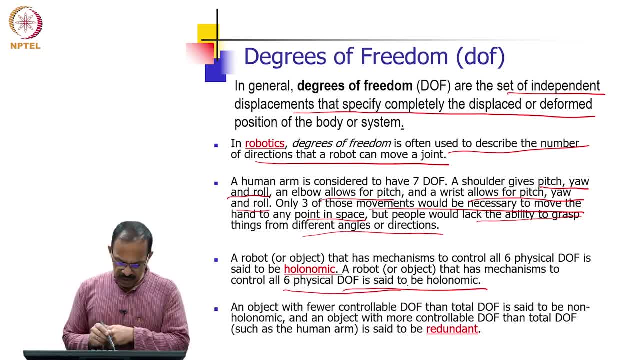 is defined. Now, an object with fewer controllable degree of freedom than total degrees of freedom is said to be non-holonomic. Suppose an object has got, suppose something has got, only four degrees of freedom, and if we can control all those four degrees of freedom, then we call: 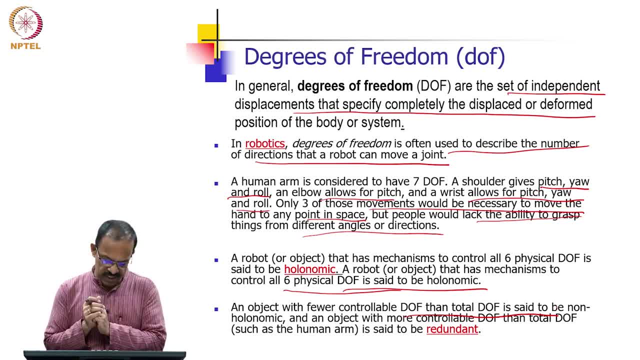 it as holonomic. Suppose: the controllable degrees of freedom is said to be non-holonomic. So if the degree of freedom is less than the number of degrees of freedom, then we call it as a non-holonomic system. And similarly, if you have more number of degrees of freedom, 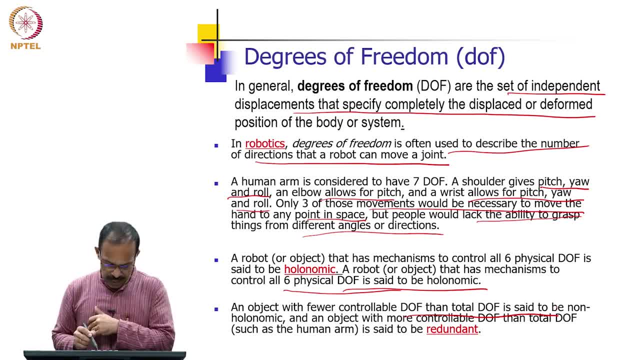 to control- I mean controllable degrees of freedom- is more than we call it as a redundant system. So that is how it is defined: if you have more controllable degree of freedom than total degree of freedom is said to be redundant. 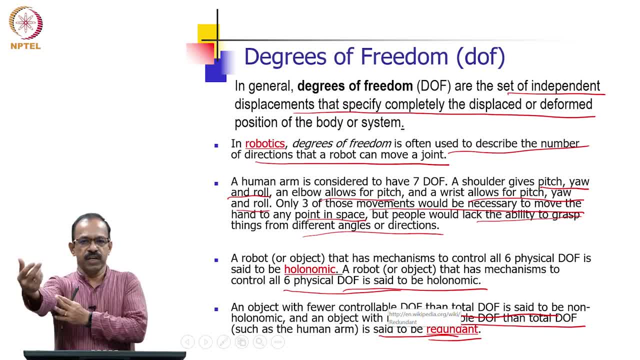 So we look at the human arm, We have got seven degrees of freedom, but to control this object in space we need only six degrees of freedom. The freedom is set to be a six degrees of freedom because it has got only 6 degrees of freedom, but we have 7 degrees. 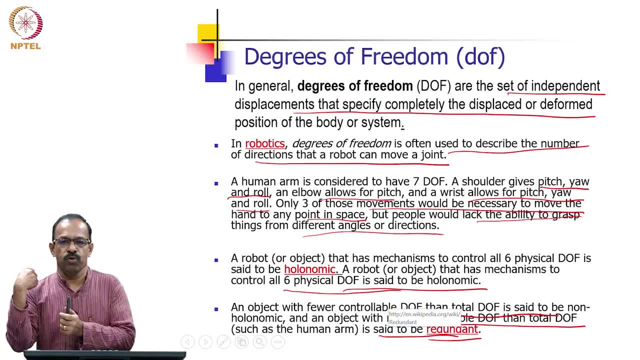 of freedom to control it. So therefore we call it as a our human hand, as a redundant system. So that is the way how we define this in the, in robotics, So we can have holonomic system, non-holonomic systems and redundant systems. 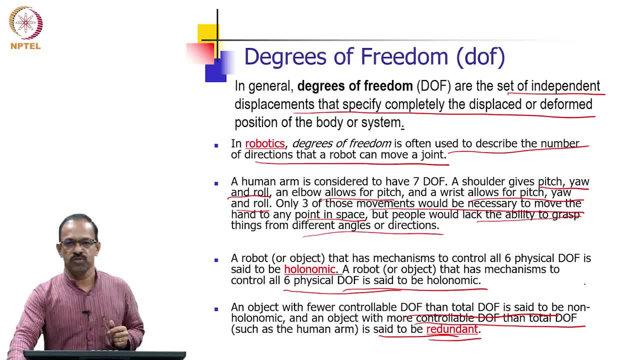 Let us look at for robotics in the in the case of robot. So we know that this positioning is done by the three joints at the shoulder and the orientation is done by three joints at the wrist. So let us see how this is actually happening in the case of an industrial robot. 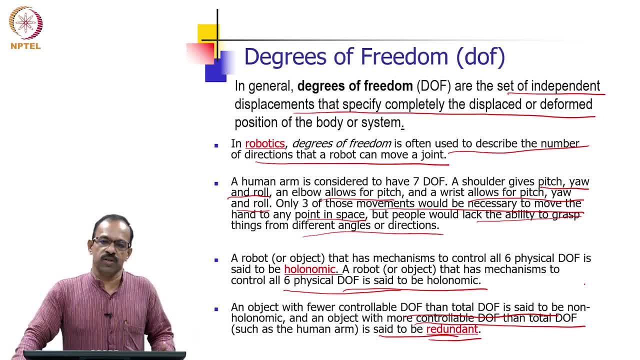 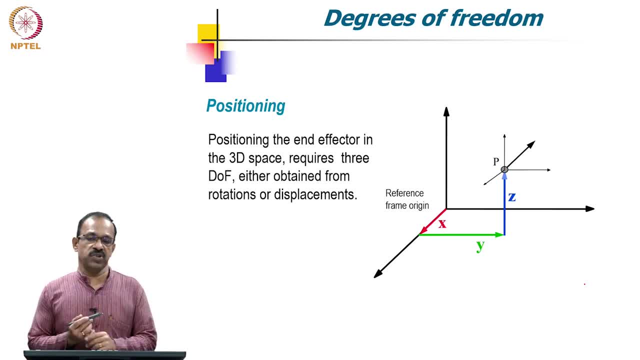 So we saw that industrial robots are used for positioning and orienting the object and therefore we need to have the 6 degrees of freedom in space. Now, if you look at the positioning of the object using a robot, the positioning of the end effect in the 3D space requires 3 degrees of freedom, either obtained from rotations. 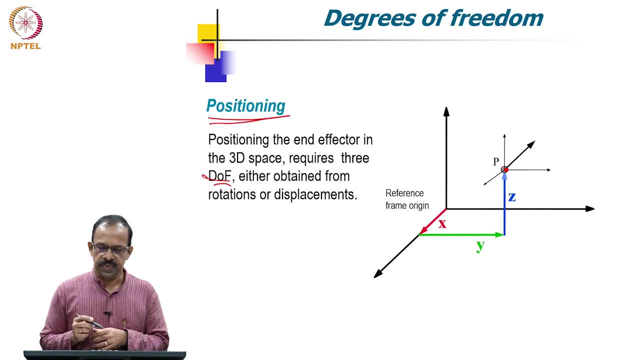 or displacement, So we can actually get position this object in space. Because what we need is positioning in x, y and z, So this can be done by 3 degrees of freedom. So the first 3 degrees of freedom of the robot will be normally used for positioning the. 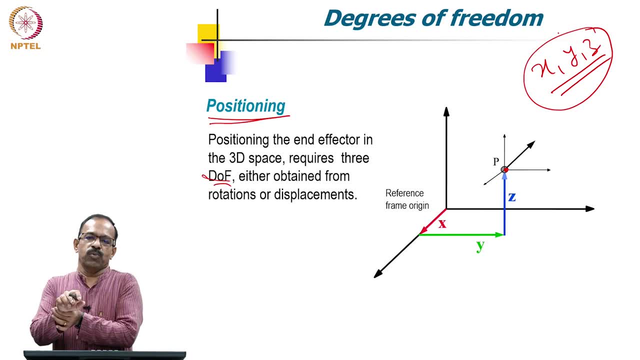 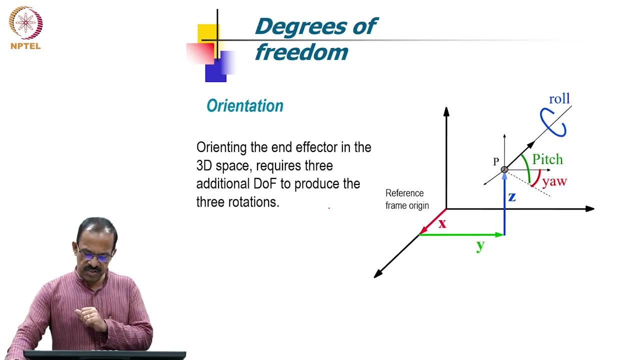 object in the space or positioning the wrist of the robot in space. So that is how we get the first 3 degrees of freedom for positioning. Then we can use, get the orientation at the tip. So this tool, I mean the wrist, if there is a wrist, and then you attach a tool to this. 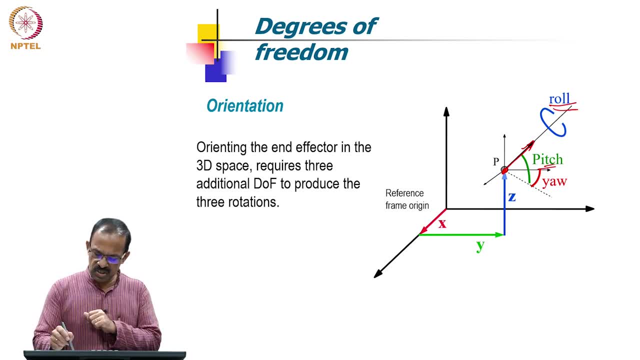 then this three orientation, that is, the role, Roll, pitch and yaw, as I told you this with respect to x, y, z axis, So you can actually say this is the pitching motion and this is the yaw motion and this is the roll motion. 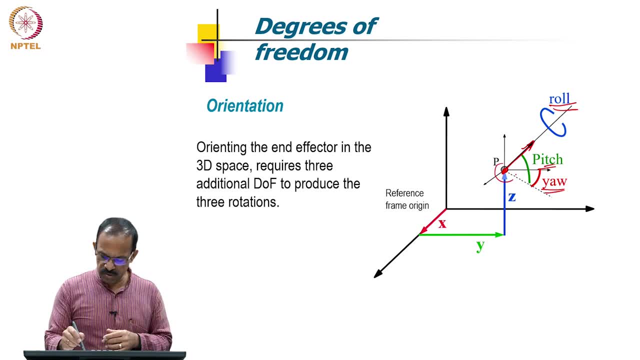 So this roll, pitch and yaw can be obtained by using another 3 degrees of freedom. So the 3 degrees of freedom of the robot will be used for positioning, or the 3 joints of the robot will be used for positioning and another 3 joints of the robot will be used. 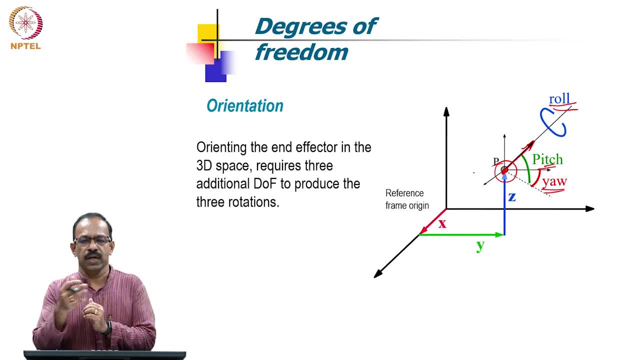 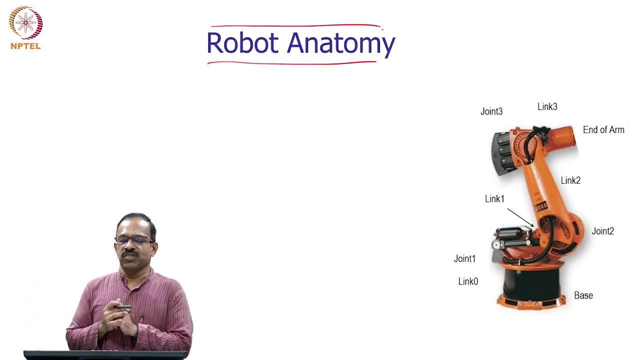 for orienting the object or the orienting the object Or orienting the end effector in the 3 dimensional space. So positioning and orientation can be obtained by 3 plus 3 degrees of freedom. So now we look at how these 3 plus 3 degrees achieved in the robot. 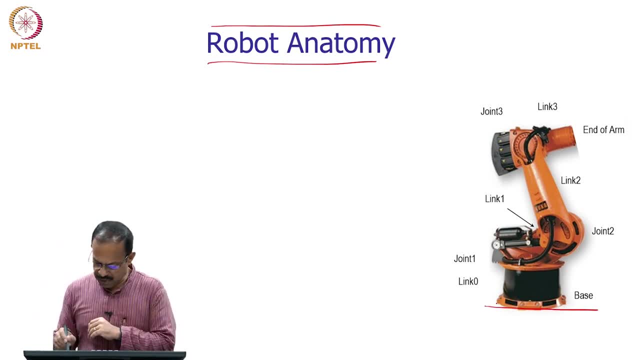 So, as we, as you know, the robot will be something like this: You have a base and we call this as the link 0, that the base is considered as a link 0. Then you have a joint attached to this link. I mean, this is the link. 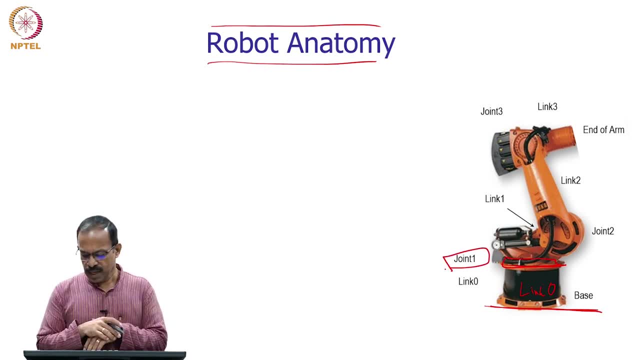 And this one base 1, that is the joint 1.. And then you have a link 1 between the link joint 1 and the joint 2.. So this is the joint 2.. So you have another joint here, So this joint 1 and joint 2 connected by a link. 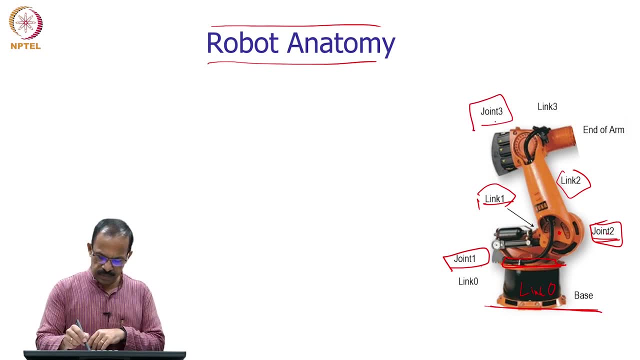 Then link 2 is connecting joint 2 and joint 3.. Similarly, link 3 will be connecting joint 4, etc. etc. So it will be going like this: Now you can see that, the joint 3.. So these 3 joints- joint 1, 2 and 3, will be used to position the wrist of the robot. 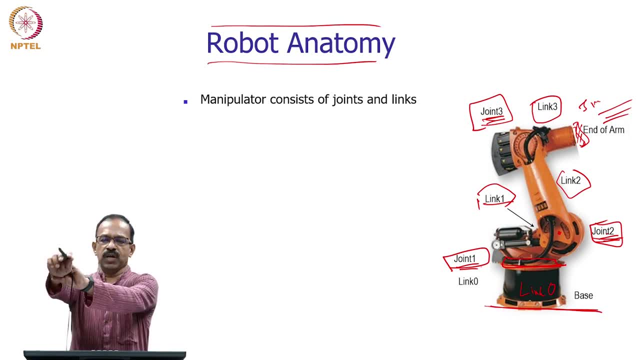 So the first 3 joints will be used to position the wrist at one point And then the wrist will be having 3 degrees of freedom to orienting it. So these are the first 3 joints- joint 1, joint 2 and joint 3- that can be used for positioning. 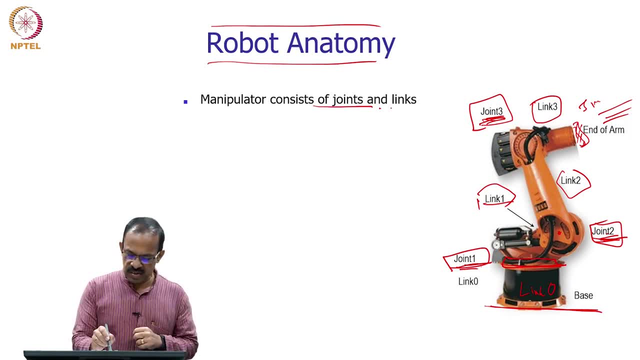 So, as I mentioned earlier also, there will be joints and links in the robot And these joints provide the degree of freedom. So each joint will be giving one or more degrees of freedom. So normally there will be having only one degree of freedom per joint. 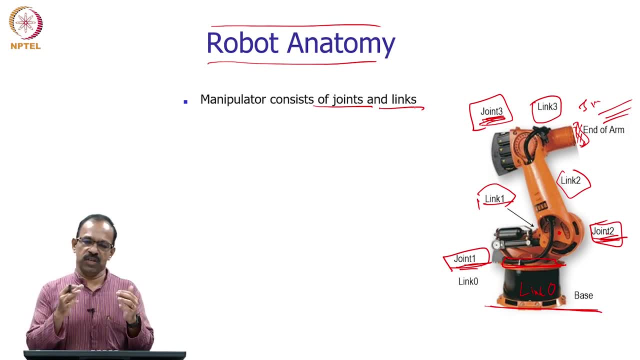 That is why it is a when you have 6 degree of freedom, unless known as 6 joint or 6 axis robot or 6 joint robot like that. So you will be having joints and links and the first 3, joint 1, joint 2 and joint 3 will. 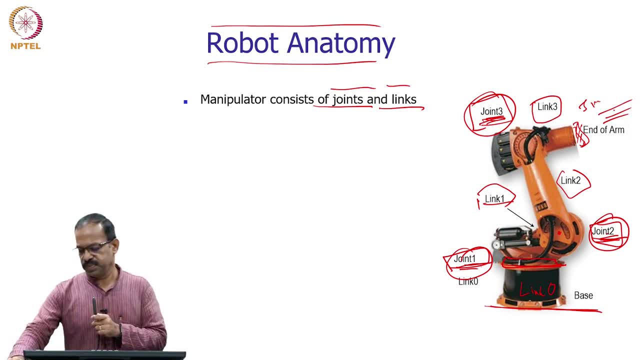 be used for positioning the wrist in the robot. So these are the 3 joints, Thank you. So the joints are supposed to give the relative motion between the links, So you can have a joint 1 which provide a relative motion between link 1 and link 0.. 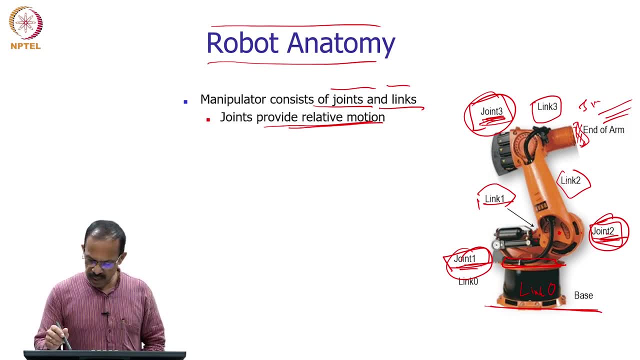 Similarly, joint 2 provides a relative motion between link 1 and link 2.. So joints provide the relative motion and links are the rigid members between the joints. So we call these as the links because they are the rigid members. Most of the industrial robots have this. 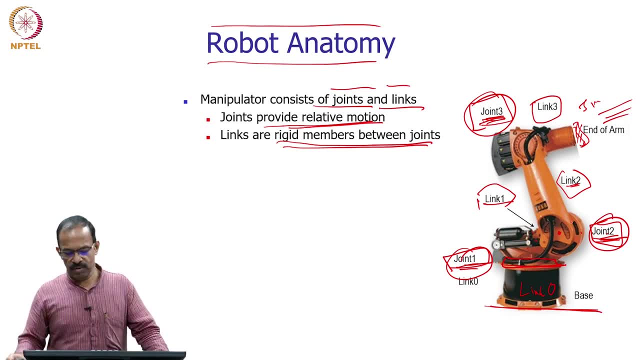 Rigid links. of course you can have flexible links also in some special cases. So this is the link which actually connects between the joints, and then that is actually a rigid element. And important point is that these joints can actually be a linear or rotary type. 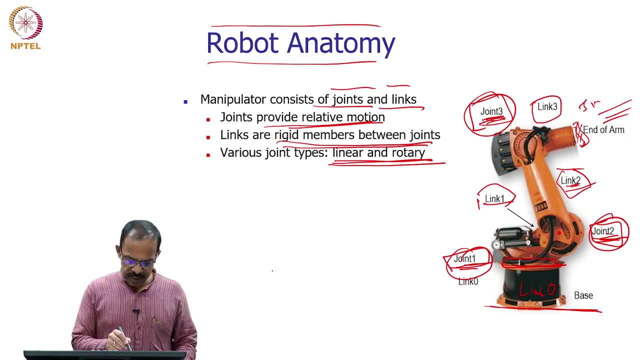 So you can have a rotary joints where there will be a relative rotation, So you can have a rotation with these joints. So this is the joint, Thank you, Thank you, So this can actually rotate, This joint can rotate and then this link can actually move. 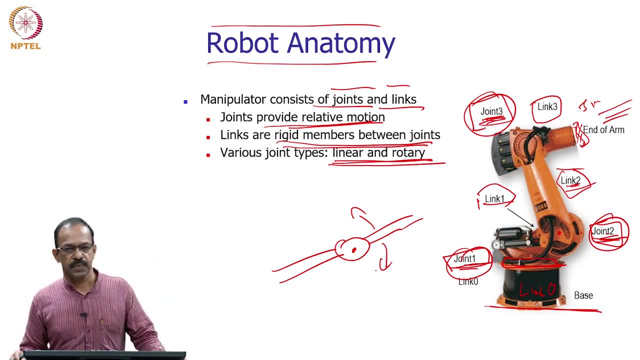 So that is the relative rotation, So that is the rotary joint. But you can have a link, prismatic link also, where actually one can actually move over the other one, This can actually move. I mean, this can actually move, the top link can actually move over. 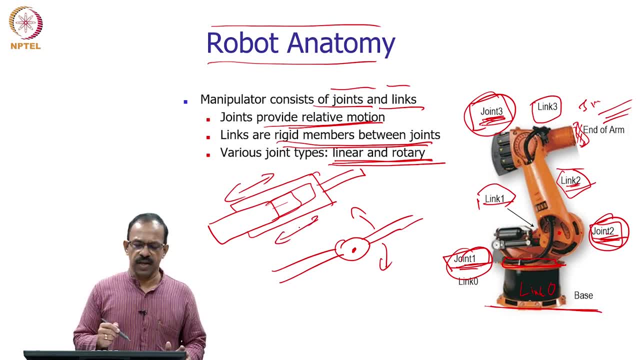 the one, this one, So you can actually have a linear motion between the links. So you can have either a linear motion, So you can have either a rotary motion or a linear motion for the joints. Whatever may be the, whether it is rotary or linear, it will be giving you the relative. 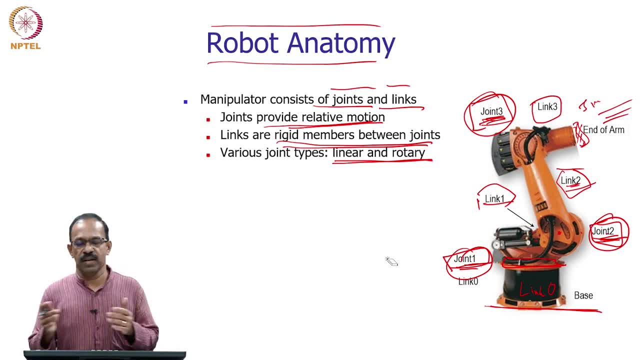 motion between the links, So the two links will have a relative motion. because of the joints, Most of the robots use rotary joints, but there are many robots which actually use linear or the known as prismatic joint also. Thank you, Thank you. 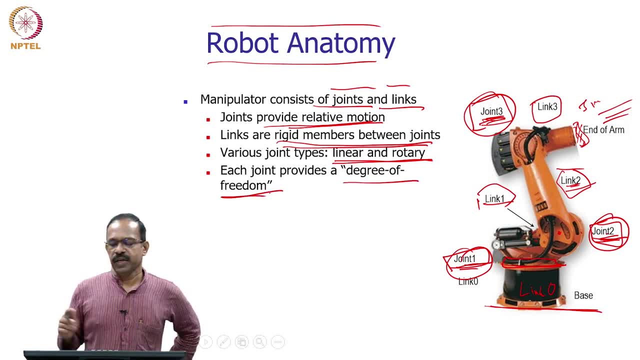 And each joint provides you the degree of freedom. each joint gives a degree of freedom for the robots, And most robots possess 5 or 6 degrees of freedom. So, as I mentioned, normally we need to have- or in general we need to have- 6 degrees of. 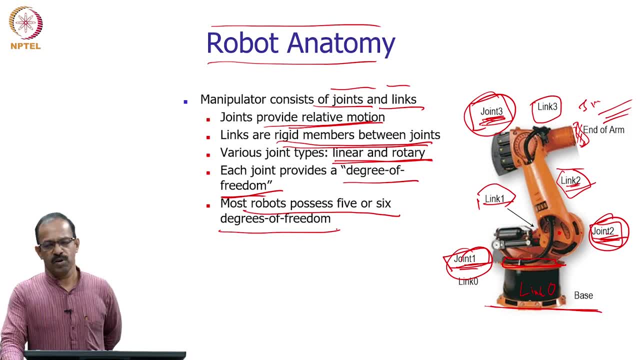 freedom to manipulate objects in space. Therefore, most of the robots will be having 6 degrees of freedom, but does not mean that we need to have always 6 degrees of freedom. depends on the application. also. Suppose I have a normal robot. Suppose I have an object which is actually moving only in one direction. 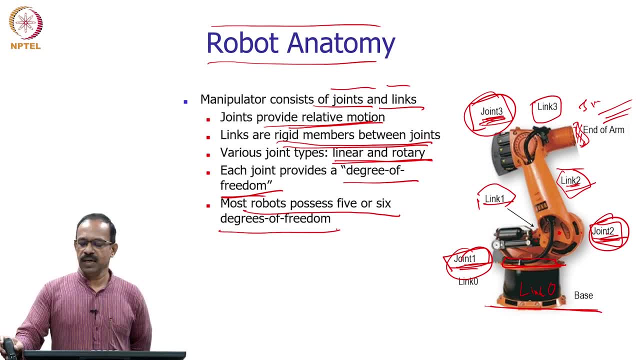 So I do not need to have all the degrees of freedom. we look at the requirement of the application and accordingly we can say that we can have a. we can have the number of degrees of freedom, So it can be 4,, 5,, 6 or you can actually have 7, also depending on what actually you want. 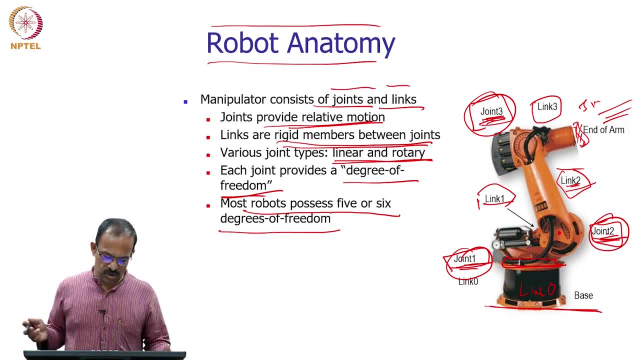 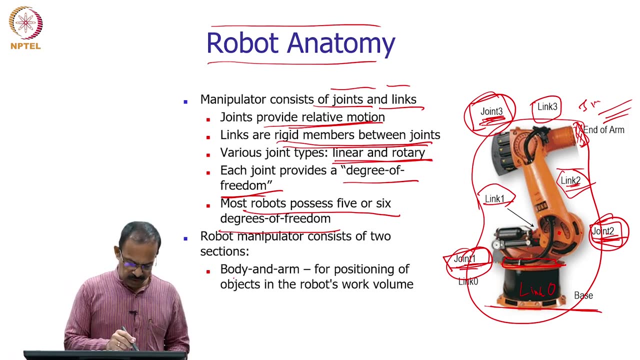 to achieve. So that is that you can have robots have 5 or 6 degrees of freedom. Okay, And as I mentioned, it consists of two sections: The first section is for positioning and the second section is for orienting. So the we call this first section, which is for positioning of the objects in the world's. 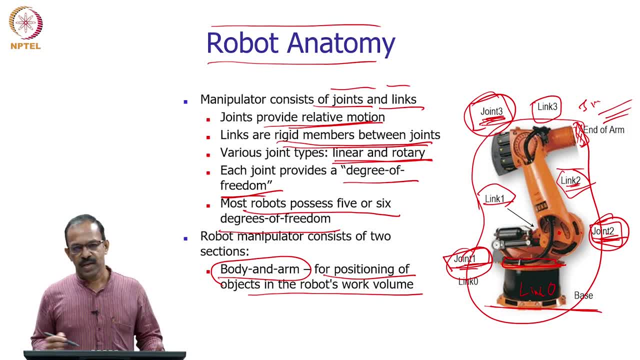 work volume. we call it as the body and arm assembly. So the first 3 degrees of freedom is used for positioning the wrist or the object in the 3D space. So that is known as the body and arm configuration. So that is the body and arm configuration. 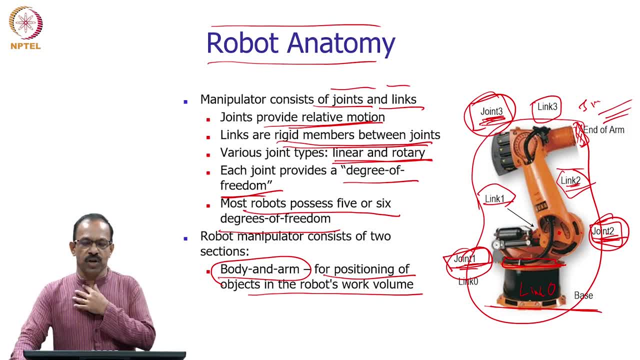 Okay, So the first 3 joints are known as the first 3 joints, endings are known as the body and arm configuration And the second part is known as the wrist assembly. That is for orientation of the objects. So the like in the human arm also. so we have up to wrist. we can say that this is we. 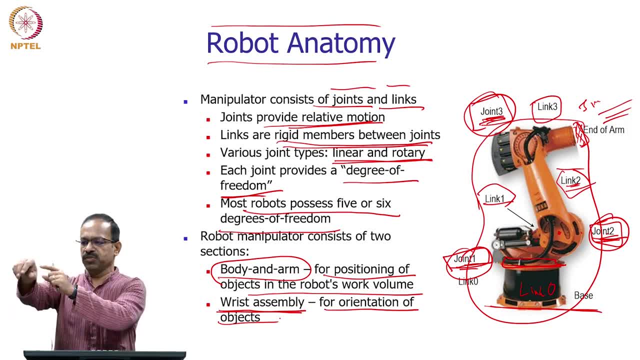 are using for positioning. So we want to position the object wherever we want using this, and then use the wrist for orienting. So it is the same way. the robot also can be classified or divided into two parts: first the body and arm, the second one is the wrist assembly. 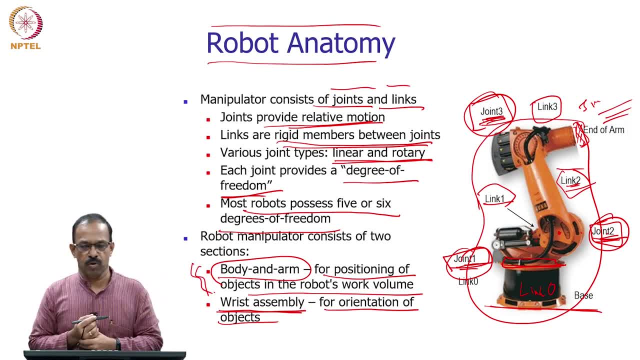 So the first 3 degrees of freedom is provided by the body and arm configuration And the second one is provided by the wrist assembly. So we have body and arm assembly and wrist assembly. So this basically provides you 3 plus 3.. So, and again, depending on the requirements, not necessarily always- it should be 3.. 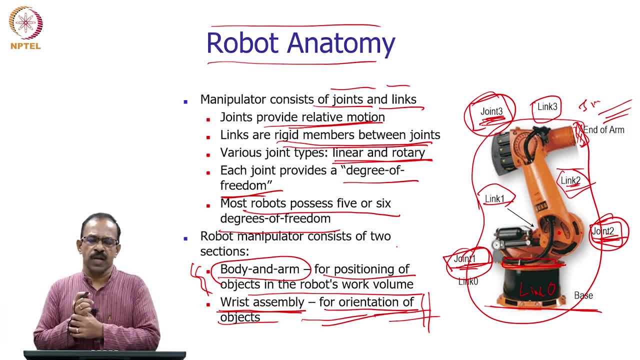 Positioning will be always 3, because you need to have position in 3 dimensional space, But orientation may not be needed in all the cases. So sometimes we will be having less space, Sometimes we will be having less degrees of freedom also, But whatever it is, the positioning part is the body and arm assembly and the orienting. 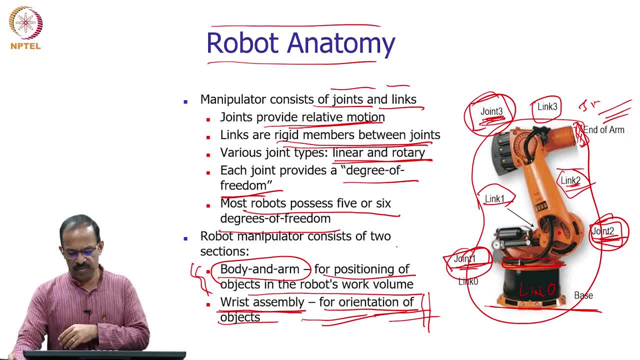 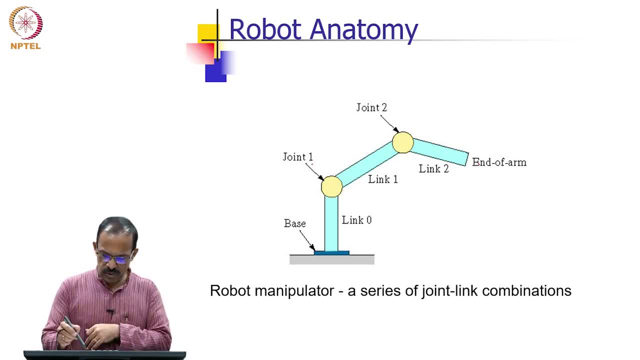 part is the wrist assembly. That is the way how it is defined. So this, actually, I already explained. So you have the base, link 0, joint 1, joint 2 and link 2.. So that is the. of course, we will be having joint 3 for the third one. 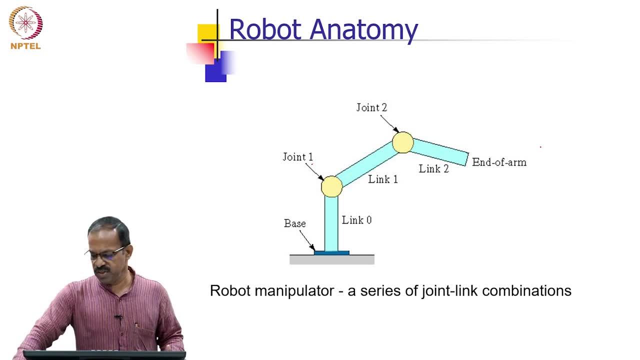 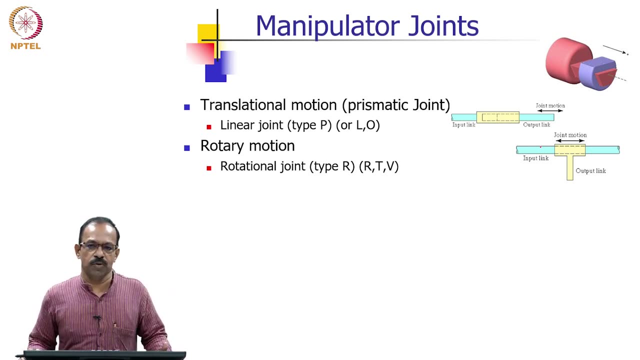 So series of joint and link combinations. Thank you, Thank you very much. Now, as I mentioned, there can be different kinds of joints. So normally rotary and prismatic are the two types of joints. So we call this prismatic as the translational motion. 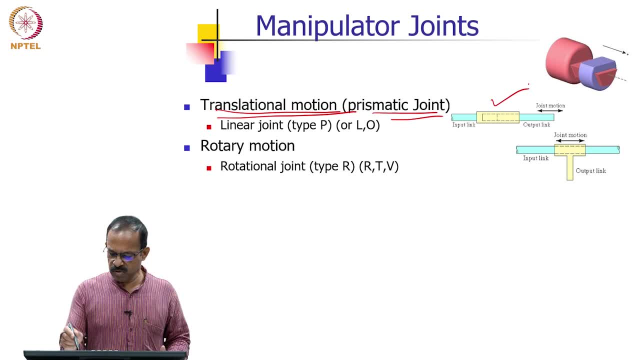 So translational or prismatic joints. So this is the example for prismatic joints. you will be having a motion, So you can have a relative motion of the link because of the joints, So there can be different ways you can actually assemble it. 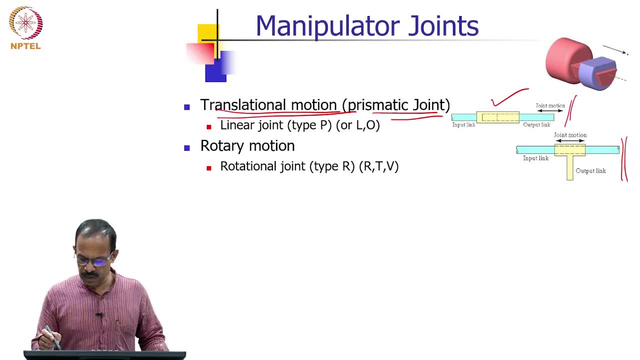 Yes, this is the one. Okay, Okay, So this is the other one. Okay, So you can actually have. this is on a PP type joint or prismatic joint, So it can be L or O. L is the linear one, this is the orthogonal one. 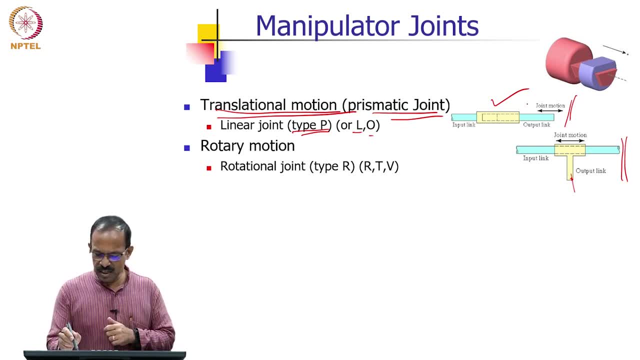 So orthogonal one is that you are getting output link. is actually this one? Here the output link is same, similar, same axis. that is why it is different, But otherwise both are giving the prismatic motion, So linear, orthogonal type. And then you have this rotary motion. 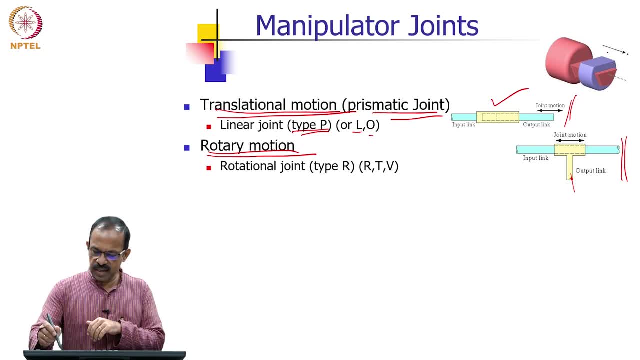 Rotary motion joints, so rotary. this is an example for the. I mean this is the CAD model of a prismatic joints. Now you can have rotary joints. they are normally specified as R type joints, So prismatic is P and rotary is R. So these are the two major types of joints, R and P. 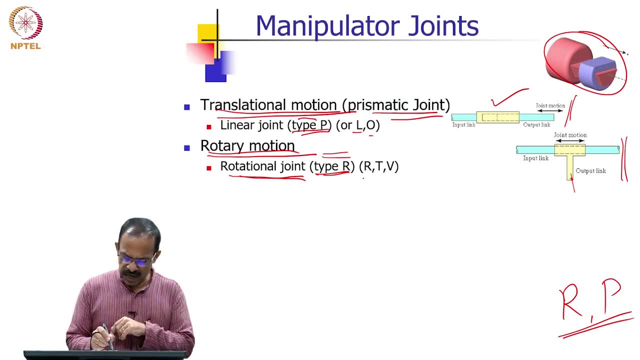 rotary and prismatic joints And within this rotary we can have variations. So I mean again, I will provide the relative. So this is the relative motion, rotary motion between the links. But the way you assemble you can actually get different motions, like you can have this. 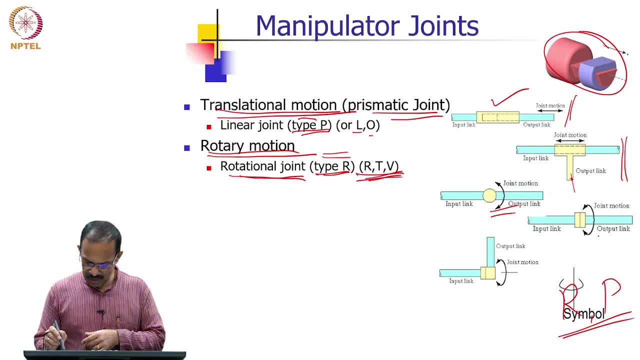 can is the normal rotary motion and this is the twist motion, and this is known as a revolute motion. So this, basically the way the links are assembled between the at the joints, makes the difference, And that is why you get this R, T and V joints. 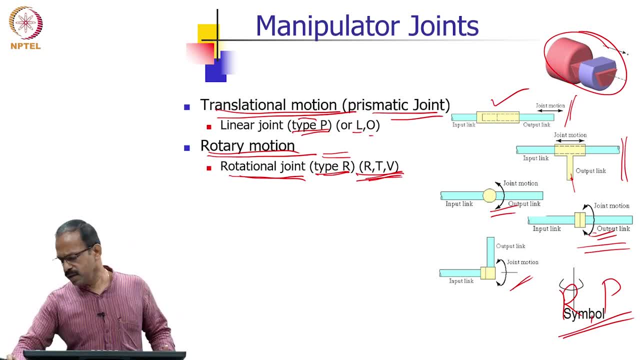 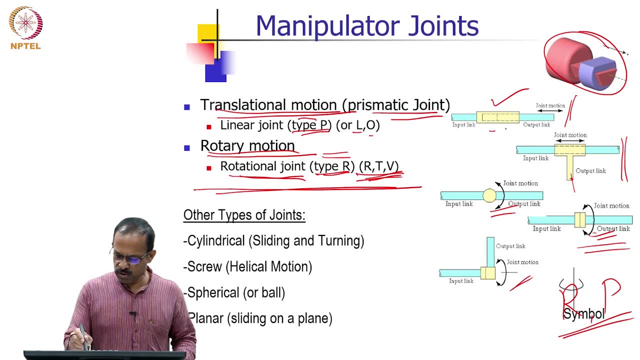 Okay Now, these are all single degrees of freedom, So you can see that each one provides you one degree of freedom. each one is one. relative motion is possible. Okay Here, whether it is rotary, twist or revolute joints, you will be getting the same kind. 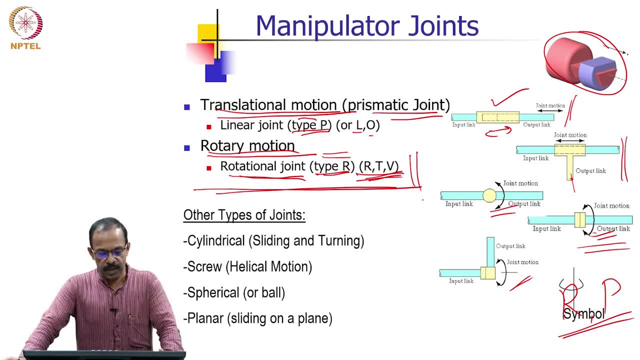 of I mean one degree of freedom. Now you can have other types of joints also, that is, you can have a cylindrical joint where you can have a sliding and turning. So that actually gives you two degrees of freedom, can actually move one sliding and. 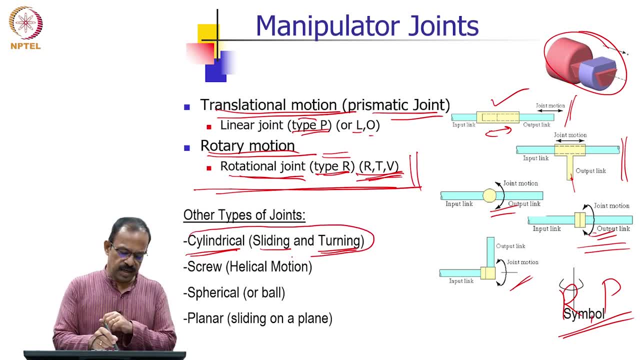 one turning. that kind of joints are known as cylindrical joints. Or you can have a screw motion. a helical motion joint can be there and can have a spherical joint also. A spherical joint actually provides you three degrees of freedom because it can actually 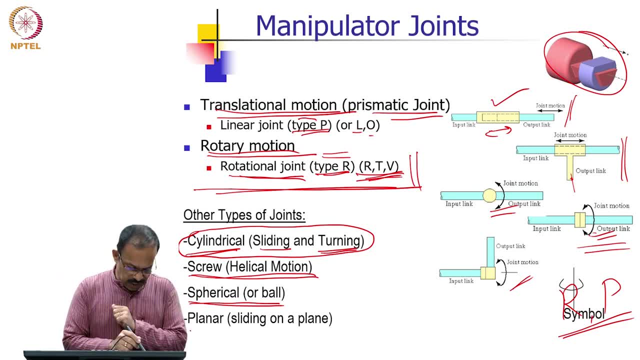 rotate with respect to all the three axes And you can have a planar one also. Again, it is a planar one. Okay, So it can have two degrees of freedom. So these are the other possible types of joints, but not really common, not used very much. 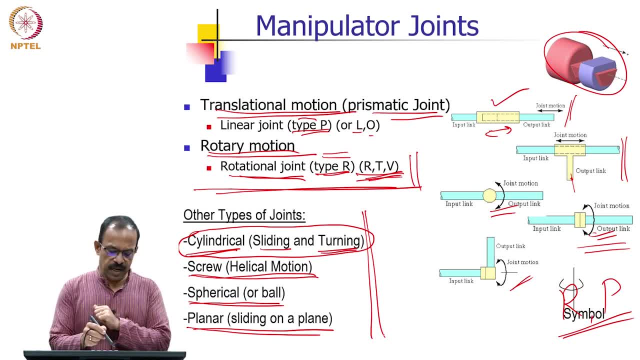 in the industry. But these are all possible. you can actually have joints of this category, also So important one, the prismatic joint and the rotary joint. So we call this. I mean these are the, these are the two major joints. 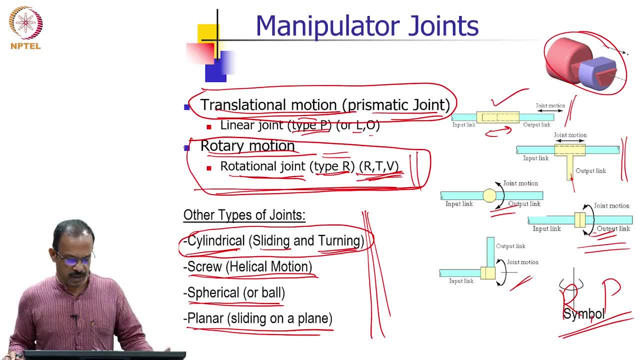 These are the major joint types that you can see in the industrial robots And the representation so it is. basically the rotary joint is represented like this. So this is the way how you represent the rotary joint. This actually shows the axis with respect to which it is rotating. 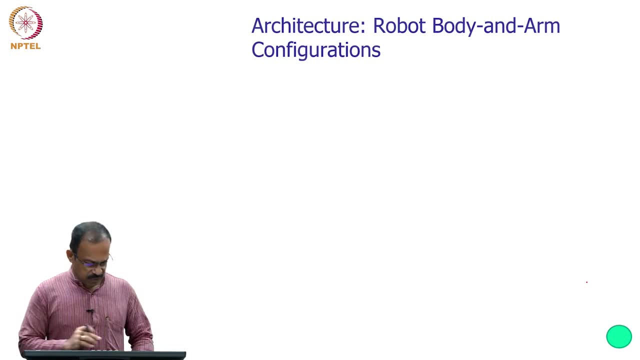 Now we mentioned about the body and arm architecture and in the body and arm architecture which is used for positioning the robot. So that is the first three degree of freedom which is used for positioning. Now the robot architecture are classified based on this body and arm architecture. body. 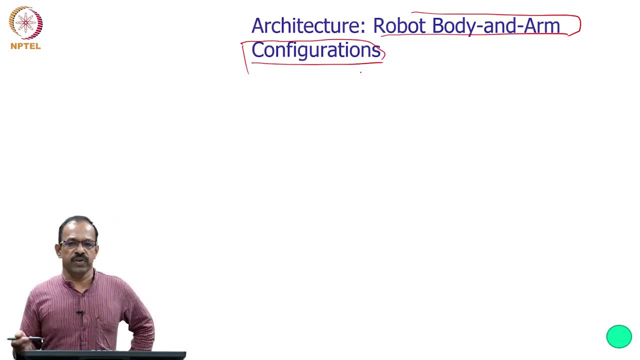 and arm configuration. By assembling these three joints- first three joints- in different ways, or choosing the type of joints in these first three joints, you will be able to get different architecture for the robots. Okay, So let us see what are the different architectures possible and how these architectures leads. 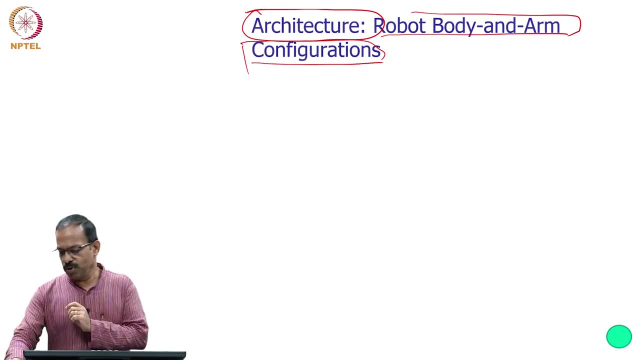 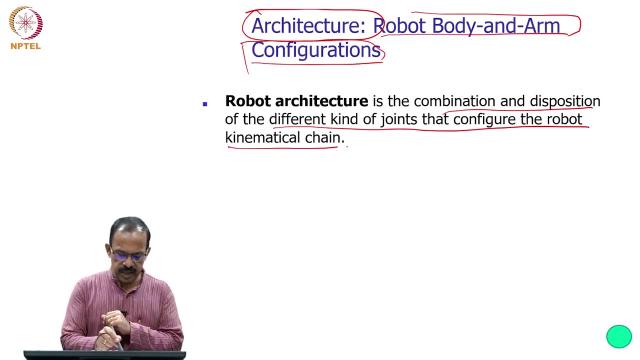 to different types of robots. So it is a combination and disposition of different kind of joints that configure the robot kinematic chain. So the kinematic chain, that is the assembly of the joints and links, makes the robot configuration And since we have multiple, I mean different types of joints. 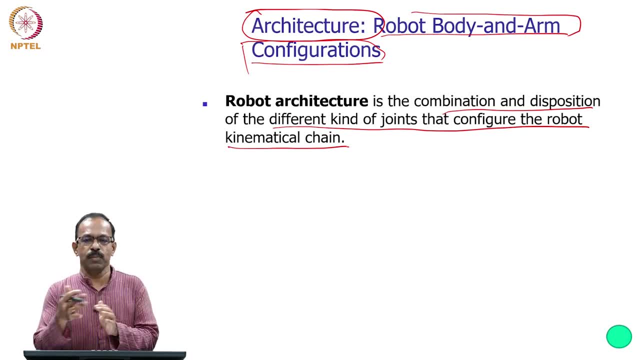 Okay. So by arranging these joints in different ways, you will be able to get different configuration for the robot, and that is known as the robot architecture. There are few commonly used architectures, So we will see what are these architectures in the in this section and see what kind 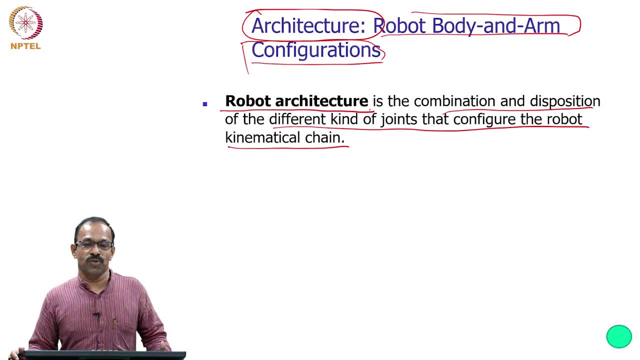 of workspace it leads to and what are the complications or what are the advantages of using different architectures. Now we know there are three joints, So the first three joints. Three joints are used for assembly, Okay, For the body and arm configuration, So that is the one which actually used for positioning. 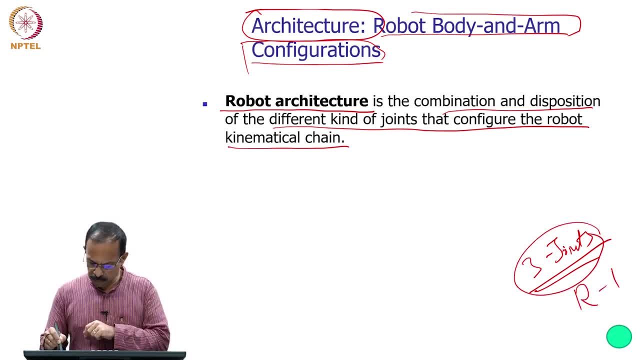 So these three joints can be either R or P. You can have either an R architecture or a R joint or a P joint, So you can have an option of having these joints in different combinations. Okay, So that is what actually gives you different architectures. 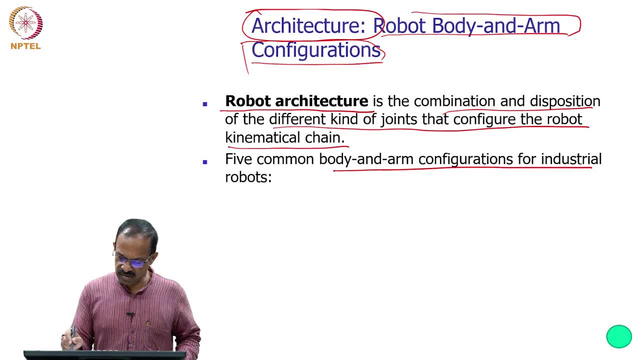 Okay, So five common body and arm configuration For industrial robots are there in the market. There are five ways actually these are arranged and that actually gives you five body arm configuration for robots, And the first one is known as a polar coordinate body and arm assembly. 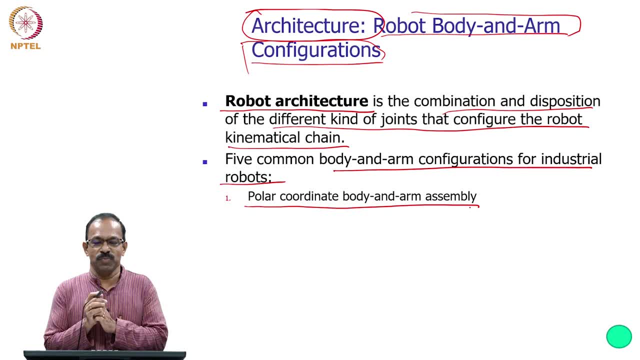 That is, you can actually represent the position of this by using a polar coordinate, and so it actually gives you configuration of R, R, P, Two rotary joints, Okay, Okay. So one rotary joints and one prismatic joints gives you a polar coordinate body and fixed. 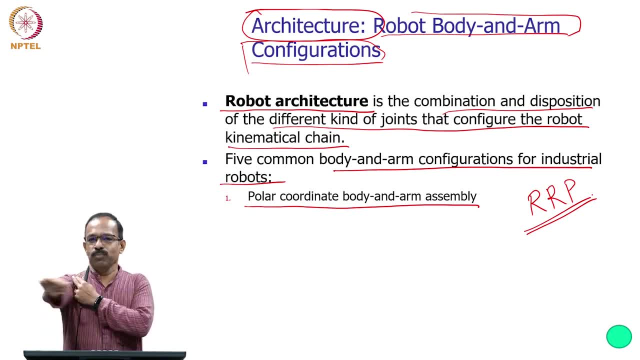 arm. So this is one rotary joints and this is one rotary motion. Okay, One rotation like this and one rotation like this, and then a motion inward or outward motion. Okay, That is a linear motion. So these three R R P helps the robot to position the tip at any point in 3D space. 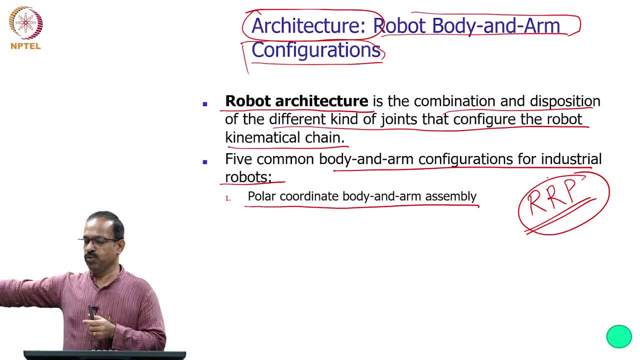 because you can actually cover this plane- Okay, And this plane using these two joints and within this plane you can actually move in and out so that you will be able to cover this and the other plane also. So this way you will be able to position the tip using these three joints. I mean R R. 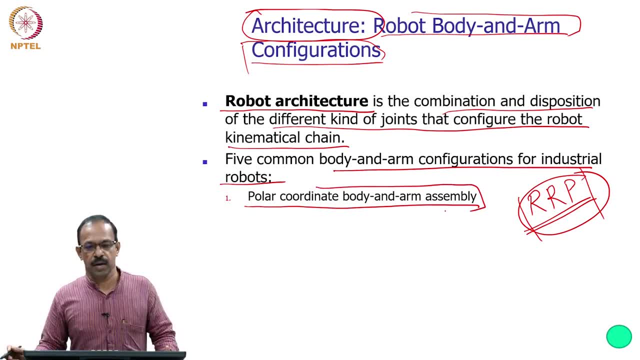 P configuration. That is known as the polar coordinate robot and arm assembly. The second one is the cylindrical body and arm assembly. So here you can actually replace one of this R with a P. Okay, Okay, Okay, Okay. So if you do a R, P, P, that is, you have a rotary joints like this which actually cover 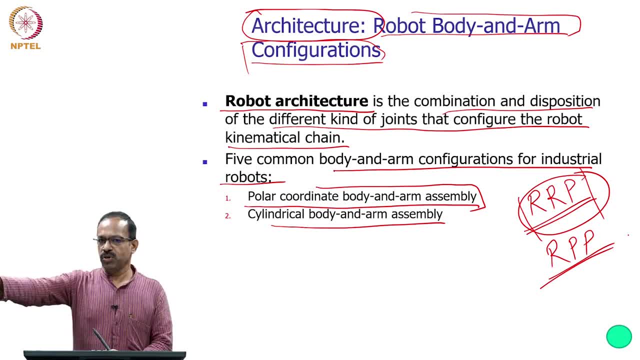 this plane and then you can actually move in and out, and then you can go up and down also, So that actually covers the whole three dimensional space. you can have R P P configuration and that is the cylindrical body and arm assembly. So you have R R P R P P. 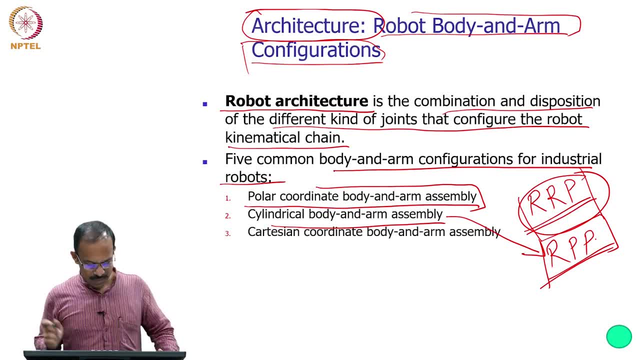 And then you can have another one Cartesian coordinate body and arm assembly which is like three prismatic joints. you can have three prismatic joints So you can go up and down, you can go side to side and then you can go in and out. also. 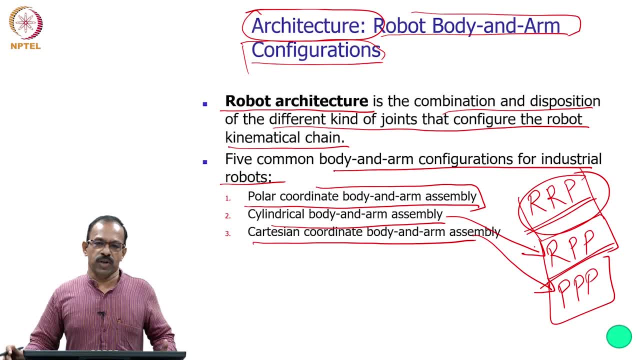 So all are prismatic joints. So you can have X direction motion, Y direction motion and Z direction motion using prismatic joints. Okay, Okay, So that is prismatic joint and that is known as Cartesian coordinate robot, Cartesian coordinate body and arm assembly. 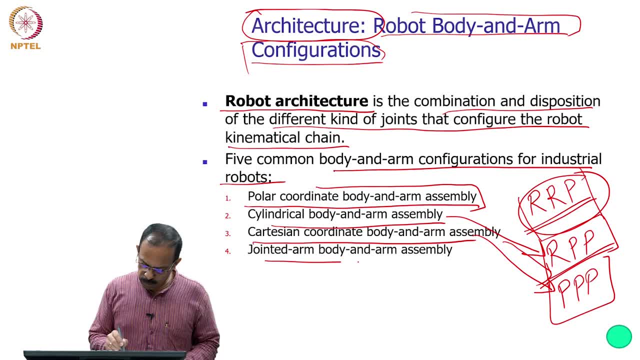 And the next one. fourth one is the jointed arm body and arm assembly, which is so this we have R R P R, P P and P P P, So the one is remaining is R R R. 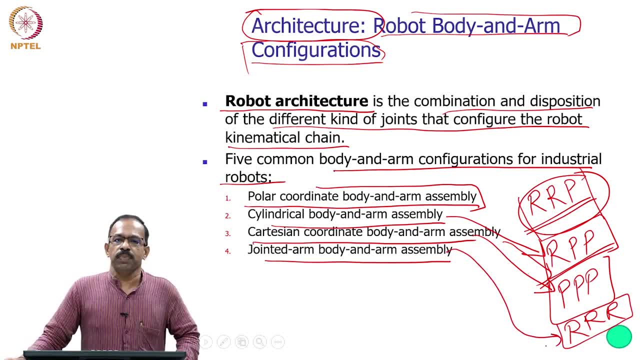 So R R, R is the jointed arm, body and arm assembly. jointed arm, body and arm assembly where? So this is all rotary joints. So most of the robots actually fall into this category. in most of the industrial robots actually fall into this category because you can have all rotations, you can have one. 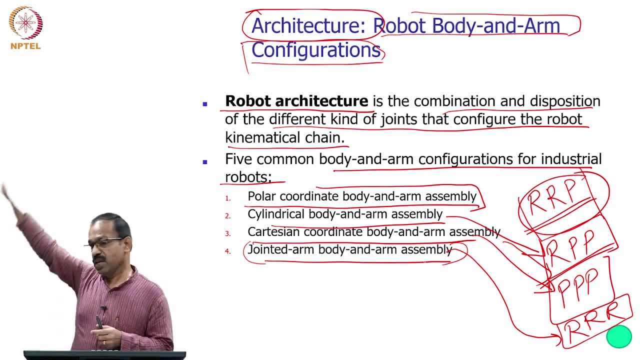 rotation here, one rotation like this. I mean you can move like this and you can have the rotation also. So you have all the three rotations possible and using these three jointed arm, body and arm assembly you will be able to get the positioning in the 3D space. 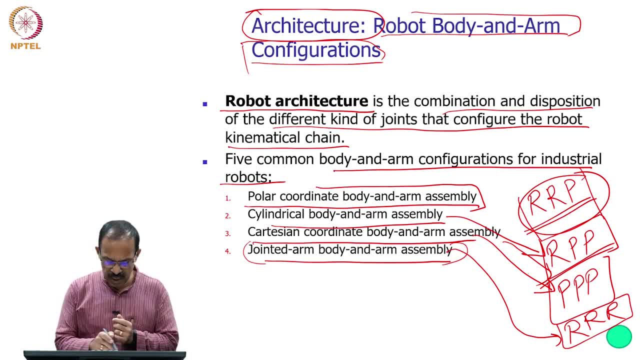 Okay, Okay. So this is the jointed arm body and assembly. R, R, R R. And the last one is a special category of robots which we call it as SCARA, So this is known as a SCARA robot, which is basically a selective compliance assembly. 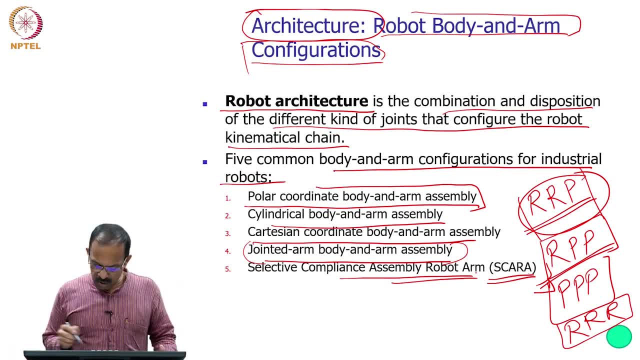 robot arm. It is actually an RRP robot. okay, so two rotary joints and a prismatic joint, So it is something like this. Okay, So it is something like a polar coordinate, but the only difference is that the joints are assembled in different ways. 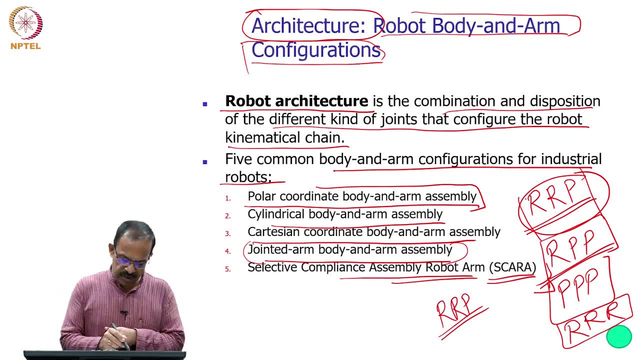 So the joint axes are arranged in a different way, So we get a different configuration, And this configuration allows you to get a compliance in one of the planes, So one plane. you can actually have a large compliance because all the motors are in a different plane. 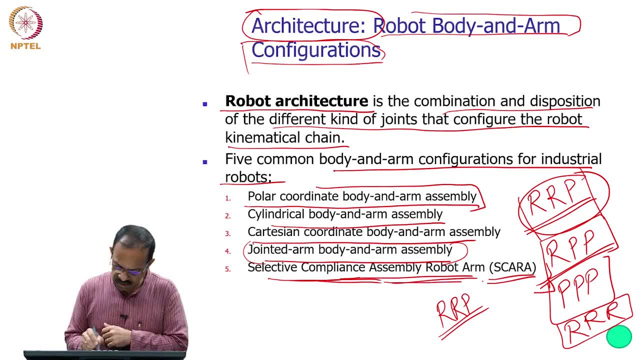 So it actually allows you to get some compliance. that is why it is known as a selective compliance assembly robot arm SCARA. So these are the five components, The five body and arm. architecture is possible using this R joint and P joint, So we use the rotary joint or the prismatic joint and then arrange them in different ways. 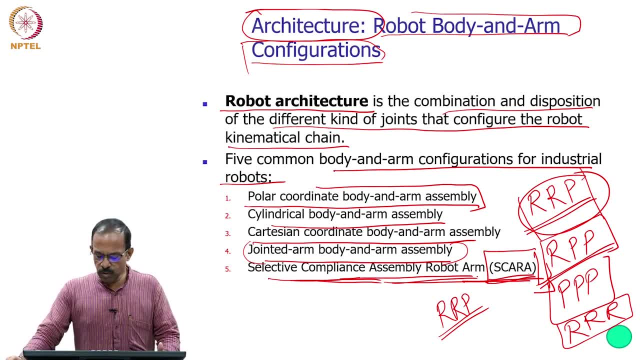 and we will get five configuration for the robots. So we will look into this configurations in detail and try to find out what are the difference between these configurations and how their workspace changes and how their kinematics get affected because of this configuration. So we will discuss this in the next class. 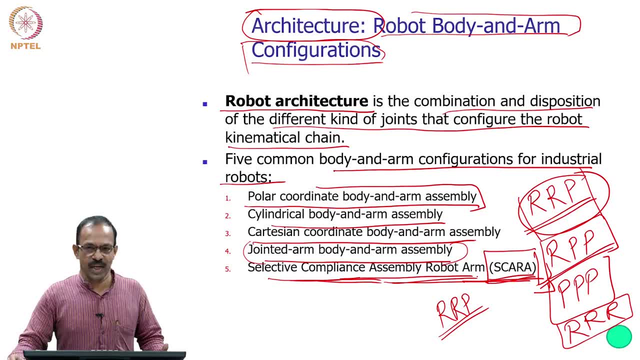 Okay, So till then goodbye, Thank you 1. 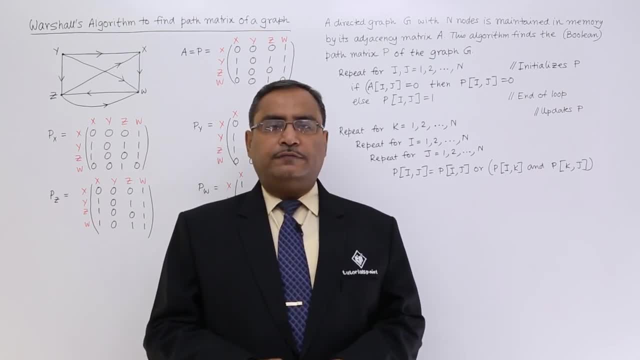 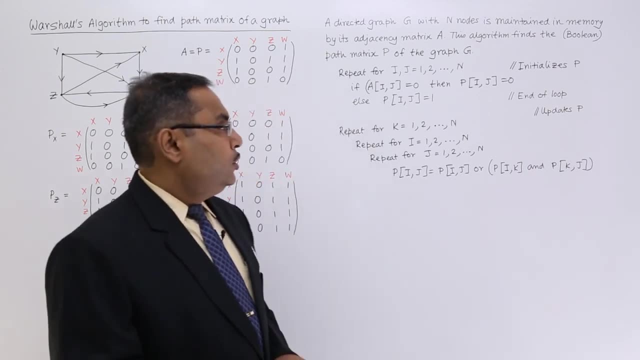 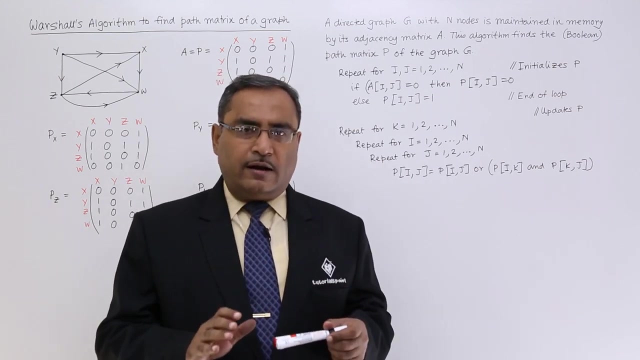 Let us consider one example of given graph on which we will be executing our Warshaws algorithm to find the path: matrix C. So this is my graph, given. This is one of the graphs we have got. There is a directed graph and here we are having four nodes actually. So 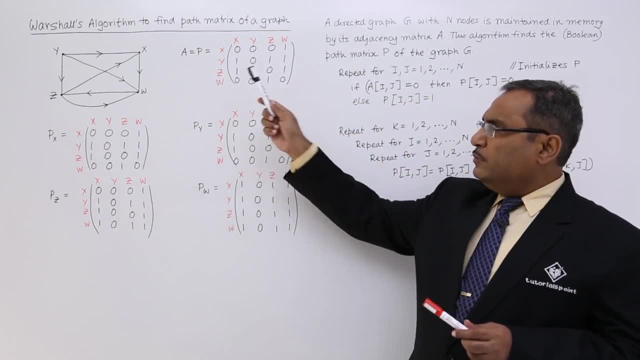 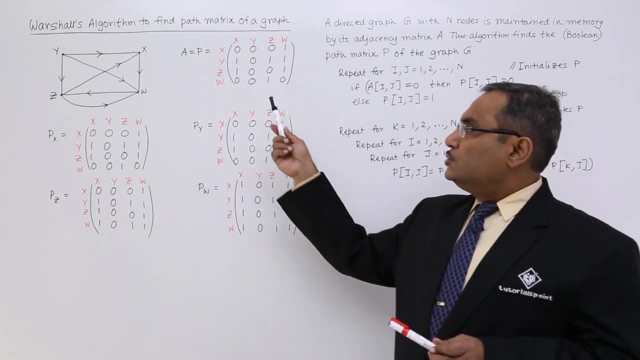 X, Y, Z and W. So from this particular graph's adjacency matrix we are going to form our path matrix in this way. So path matrix is something like this one. So from the adjacency matrix we are getting the path matrix like this: 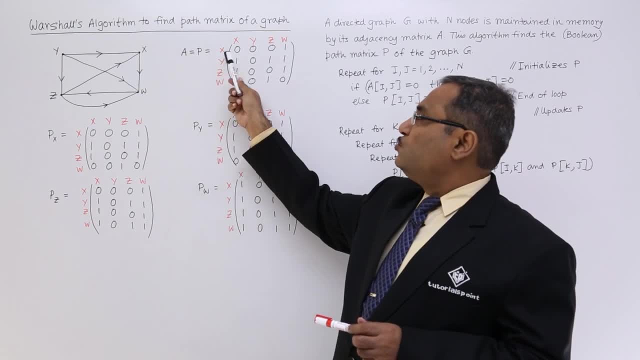 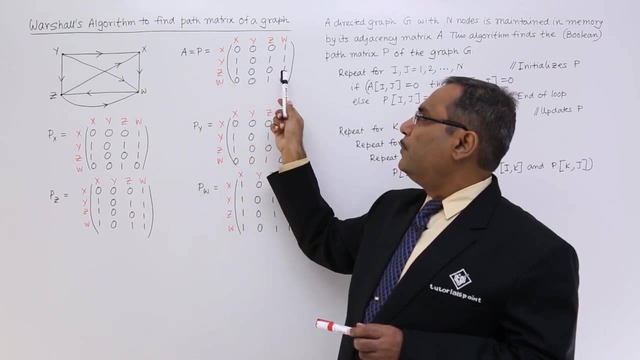 So now this path matrix depicts that from X to Y there is no path. From X to Z there is no path. From Z to Y. there is no path, but there is a path from Z to W. And if you 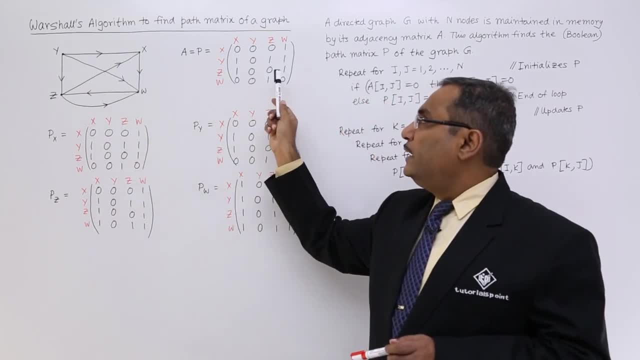 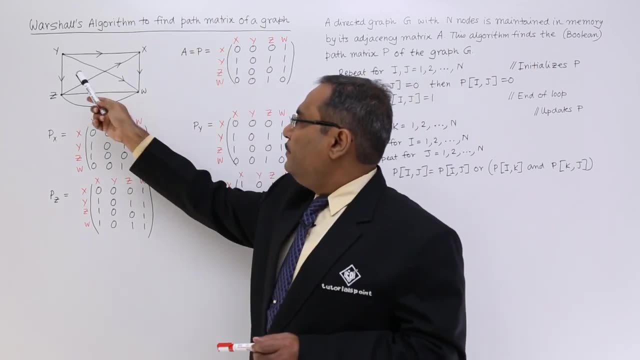 go. if you trace this path, you will see that there is no path. from X to Y, there is no path. So from this particular graph, you will be getting this one hydrological. I am just showing one or two examples, such Y to X, there is a path. Let me go for Y to X. 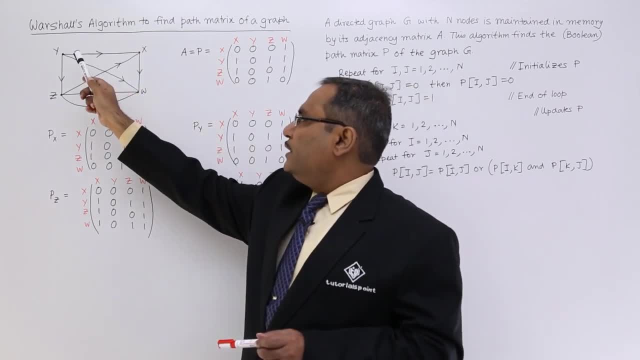 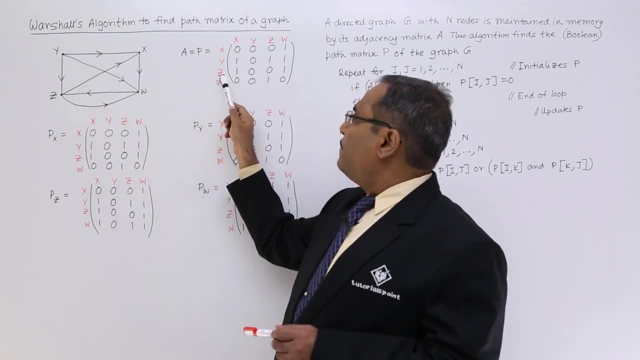 Yes, there is a path. Y to Z, there is a path. Let me check. Yes, Y to Z, there is a path. There is no path from Y to Y. Yes, there is no self loop. There is no path from Z to Y. 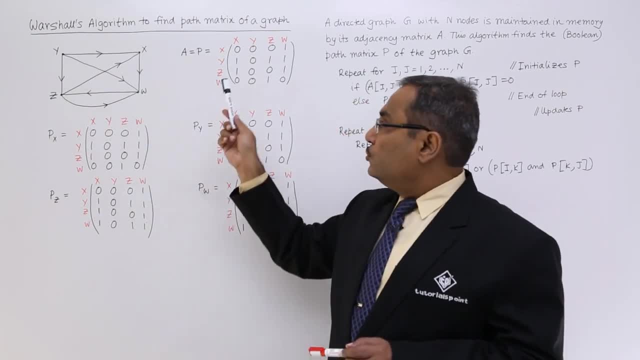 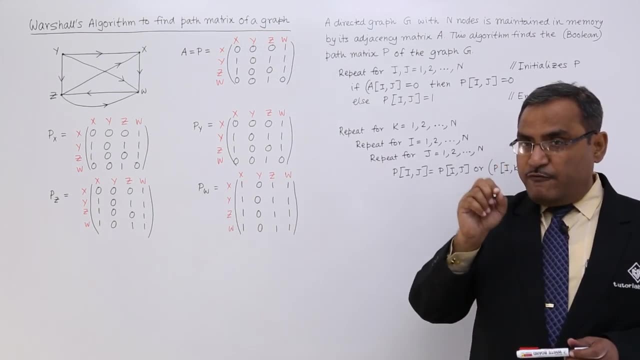 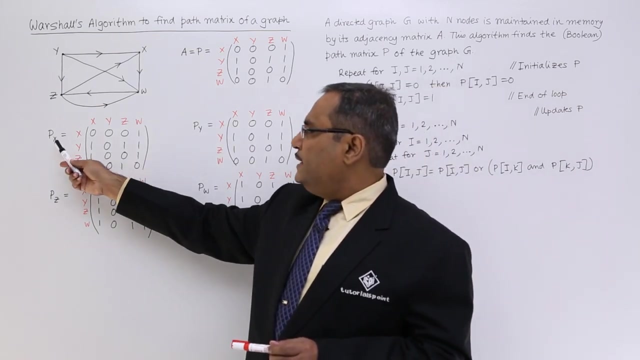 So Z to Y, Yes, from Z to Y, I cannot move. So this particular matrix is very much logical. Now we are going to take each and every node as intermediate one to generate more paths. So now, if you go for P X, if you go for P X, you see almost the same matrix we are getting. 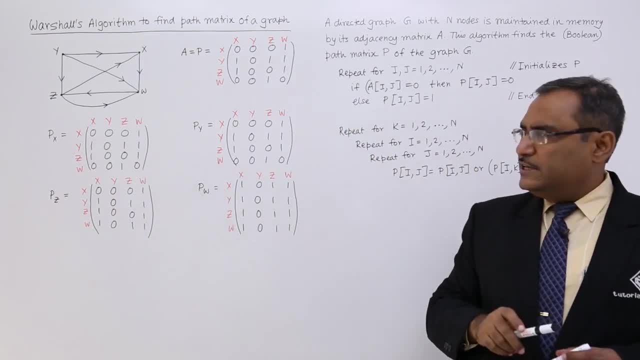 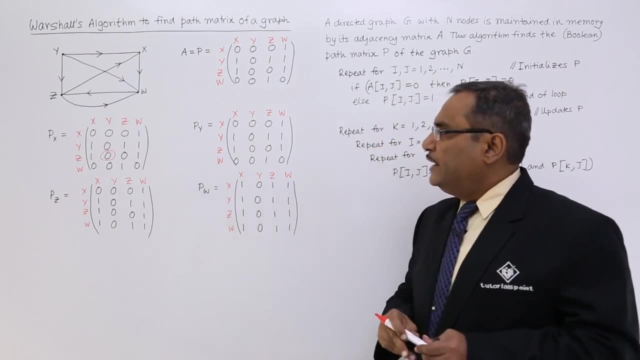 So P X could not change anything. Let me check one. So I am just for the sake of simplicity, I am just taking this one as an example. So Z to Y. Z to Y is 0.. So Z to Y is 0 means.